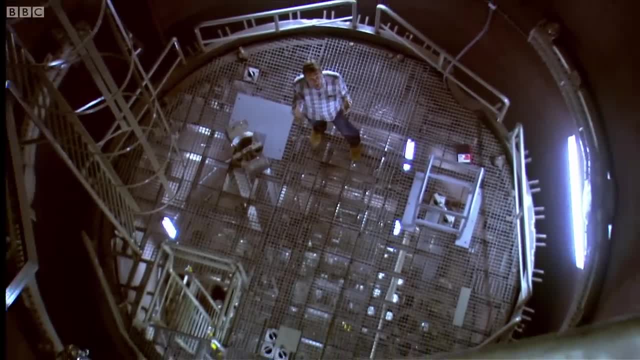 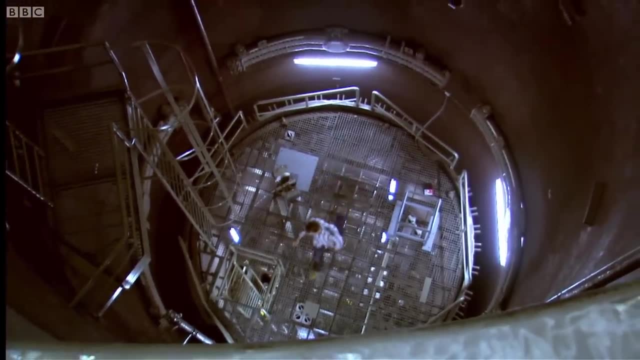 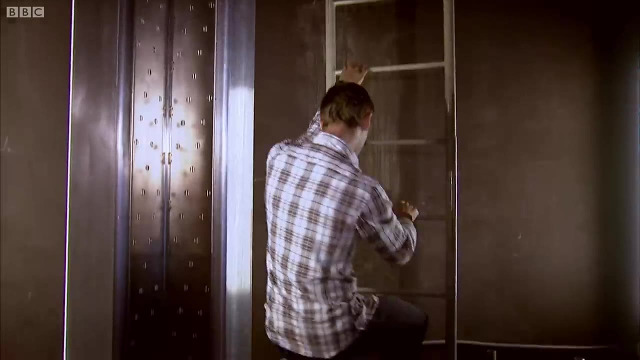 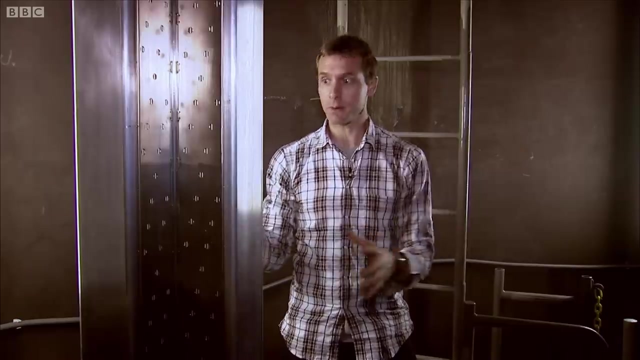 Pushing these walls apart with a force of around 40,000 tonnes, But where is all the energy coming from to do that? It's coming from down here. These are nuclear fuel assemblies. Now, if operational, this small space would be packed with over a hundred of these. 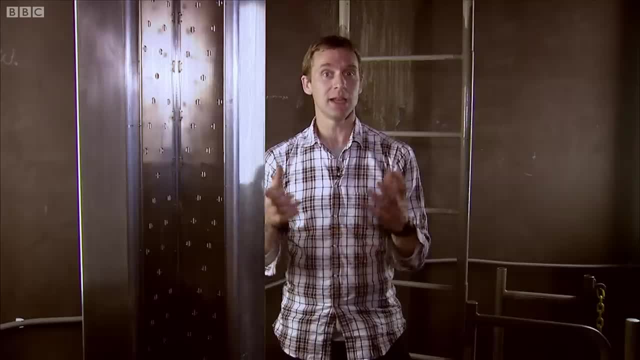 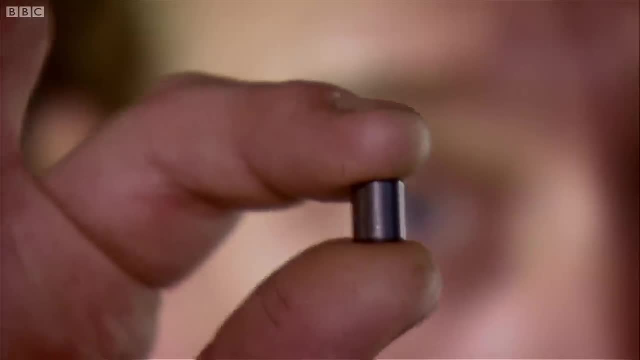 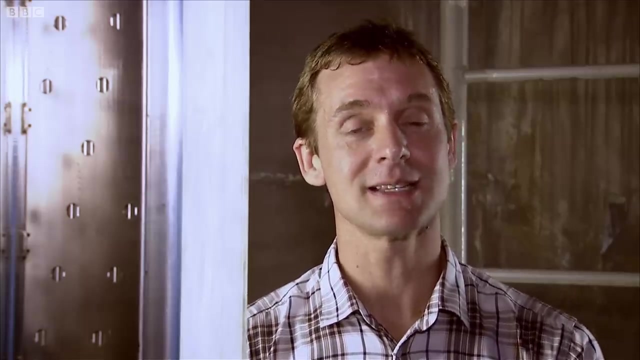 each giving out vast amounts of energy in the form of heat, And that's because every one of these square metal tubes would be packed with thousands of little pellets like this. The pellets are made of uranium oxide, And uranium is very special to us because it's an atom we can split. 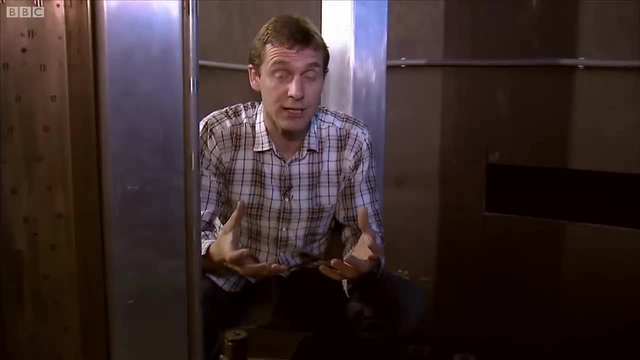 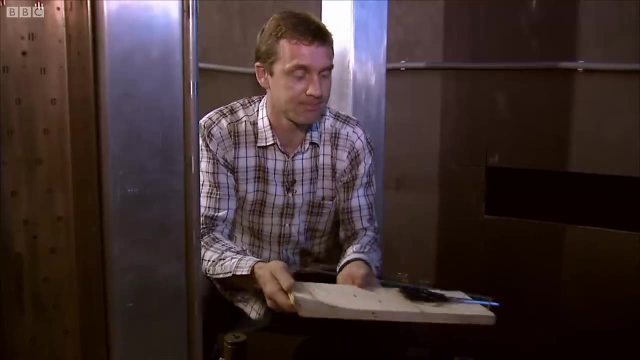 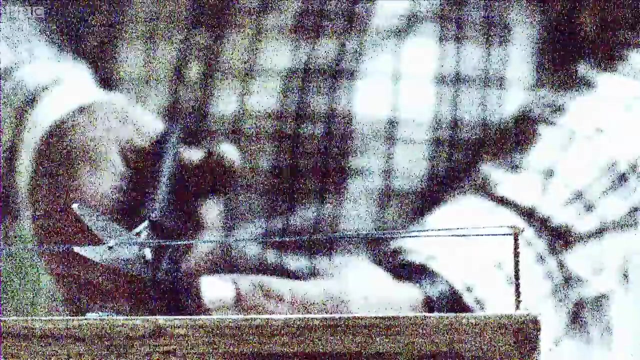 When things break apart, they tend to release the energy stored in whatever was holding them together. Now, it doesn't matter whether that's an atom or a stretched elastic band like this one, So I'm going to come in, split it, and what I end up with is two smaller high energy elements flying off in opposite directions. 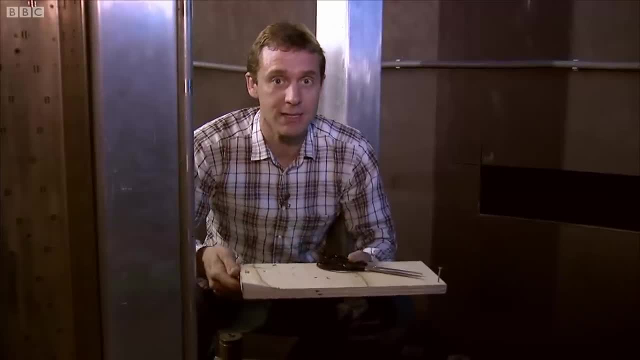 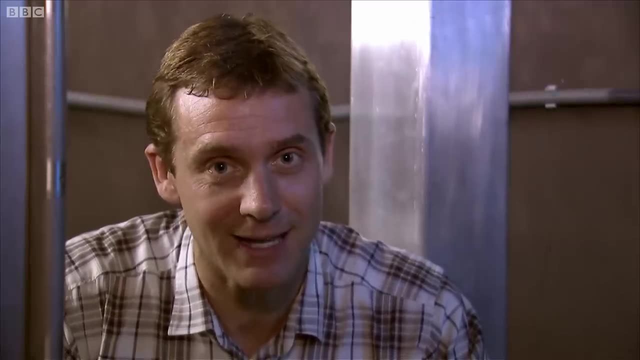 Now, when that's an atom, those two smash into their surroundings, warming things up. Big difference is, no matter how small your scissors, they're not the tool for splitting an atom. To do that, you need a small particle called a neutron. 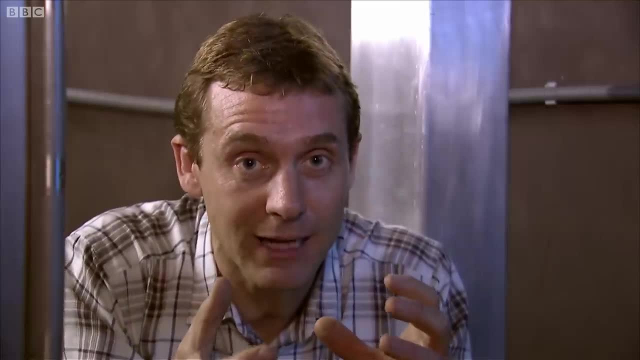 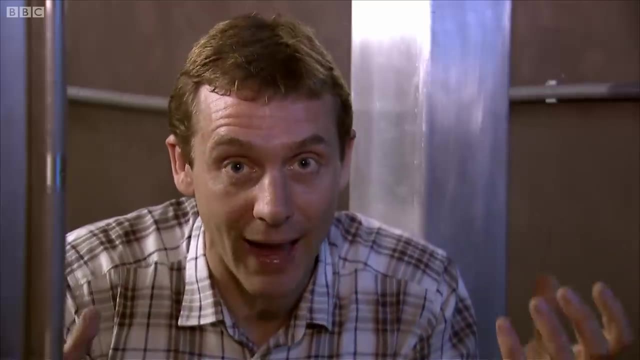 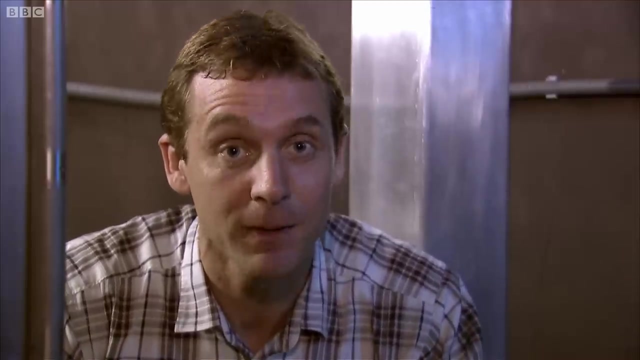 Now, when this hits the very centre of a uranium atom, it can get absorbed, causing the atom to become unstable and split. But as well as releasing all that energy, you also release two or three more neutrons that can then fly off into the surroundings, causing more trouble. 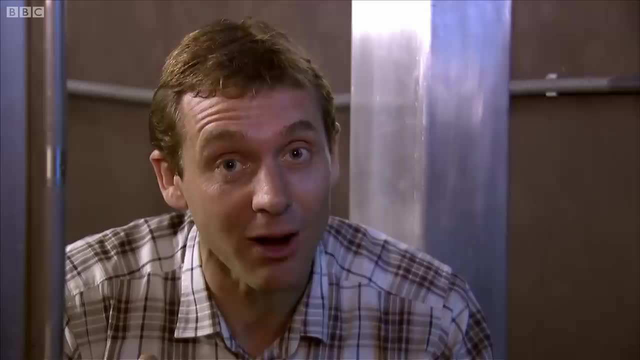 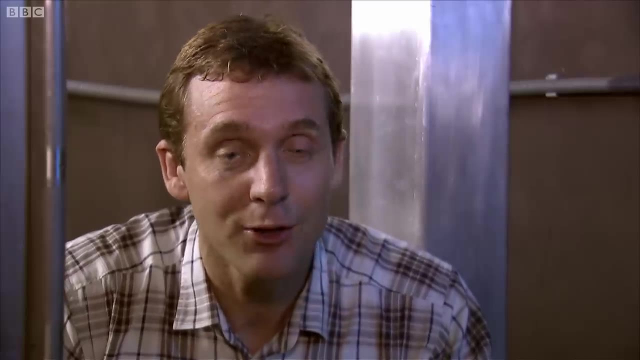 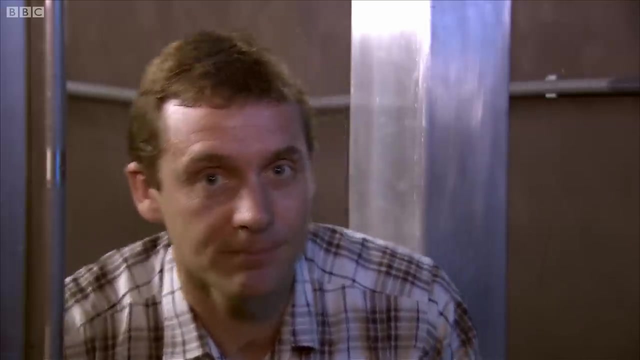 Thing is that's still not really enough to sustain a nuclear reaction, Because uranium atoms don't absorb neutrons that easily. The neutrons need to be going at just the right speed, And for that this whole reactor needs one more thing. 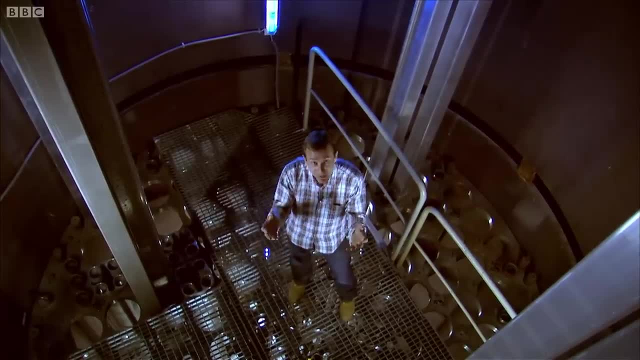 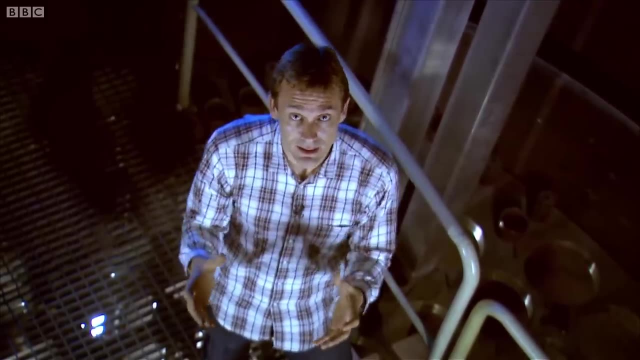 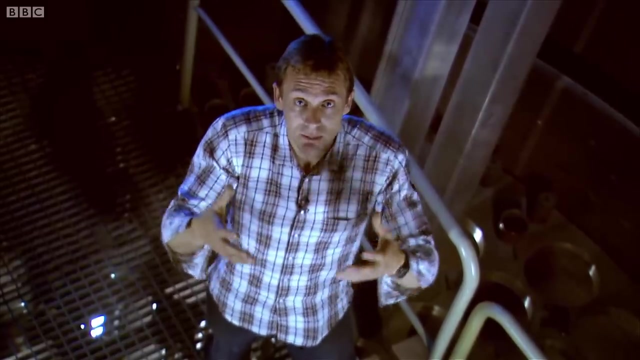 Just add water. The water plays a pivotal role because it slows down those little neutrons to a speed where they're much more likely to be absorbed by nearby uranium atoms, causing them to become unstable and release more energy and more neutrons in a continuous cascade.